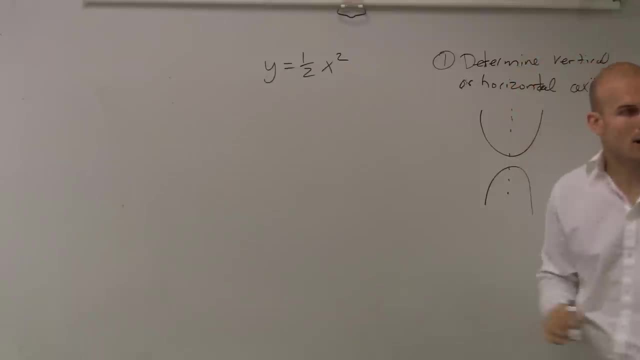 vertical line, meaning my parabola is going to equal open up or it's going to open down, all right, But it's going to have a vertical axis of symmetry. Wait, how do you know that? How do I know, for my problem. 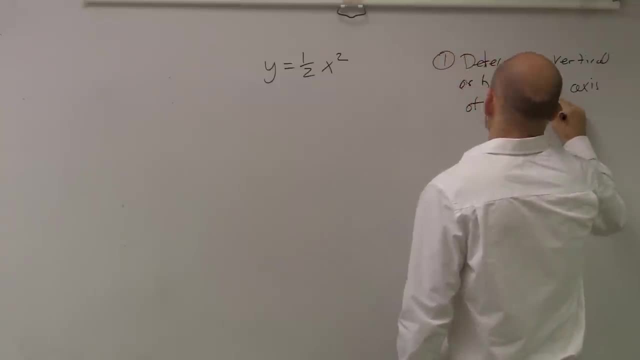 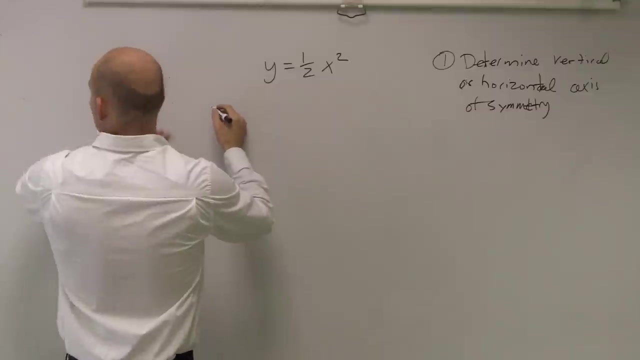 Yeah, Because I have an x squared, all right. And so we look at what happens with what's our vertical axis, What's our standard equation for a parabola that has a vertical axis, right? So the first thing I want to do is just determine if it's going to be a vertical or a horizontal. 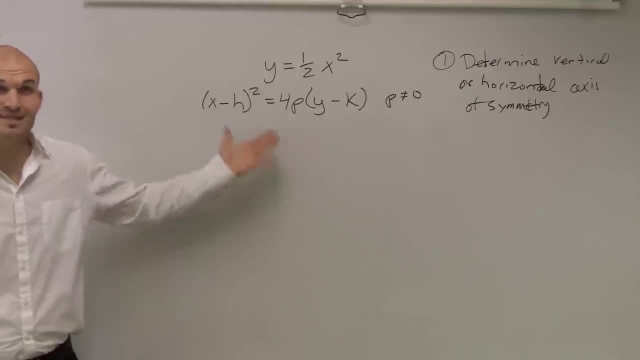 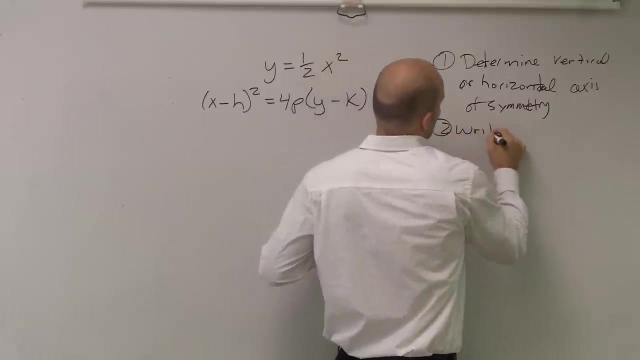 axis, If it's going to be a horizontal or a vertical. Why do I need to determine that? Because there's two different formulas, right, There's one for our vertical and there's one for our horizontal. The next thing I need to do, which I just did, is write the standard equation. 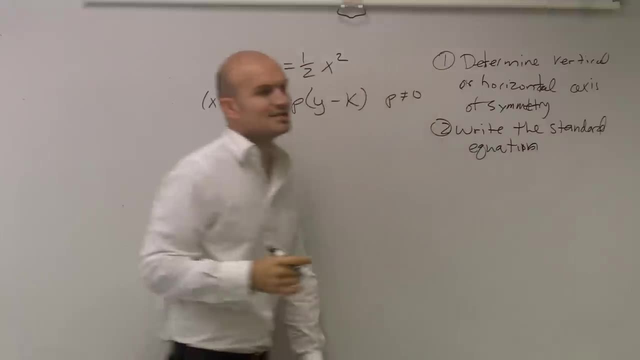 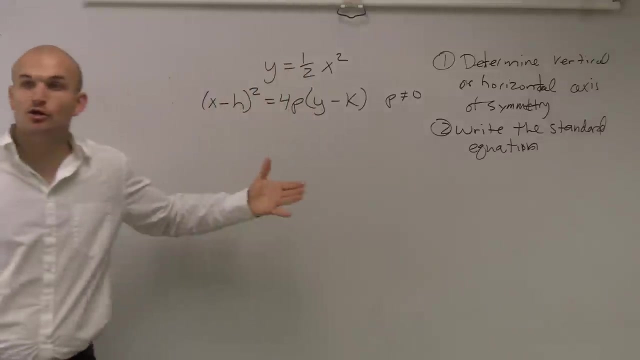 So a lot of students always want to default to one or the other. It's important for you guys to notice first off and just write it down. Hey, this is going to be a vertical parabola. It's either going to open up or it's going to open down, but I know it's going to be. 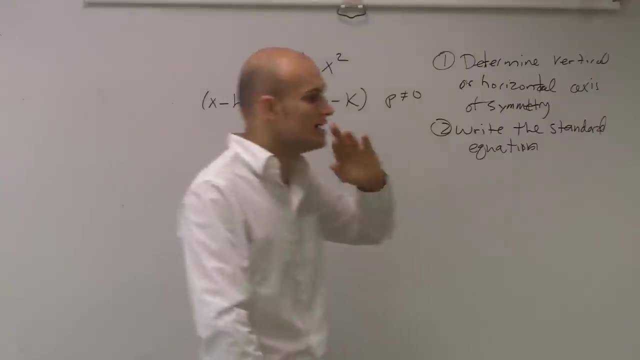 a vertical parabola. It's going to have a vertical axis of symmetry, All right, So now what we need to do is we write the equation. All right, So now I know what I need to look at. Does this problem look anything like this one? 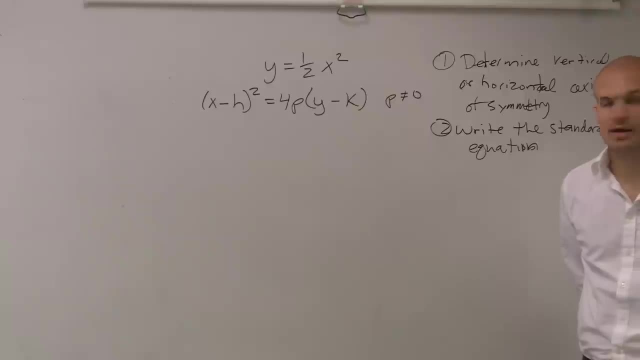 No, it doesn't. So what I want to do is: I'm sorry, I want to write that in the form. so it looks like. so it looks exactly like that, all right. So what I'm going to do is I'm going to say: y equals 1 half x squared. 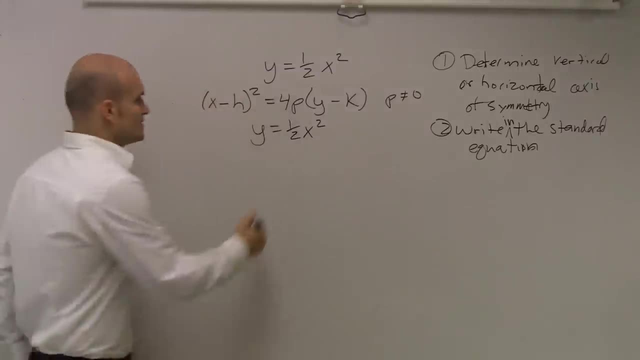 So let's put the x over there on the square. So let's swap these around. So therefore, I'll have a negative 1 half x. Let's just swap these around. so I have x 1 half. x squared equals y, right? 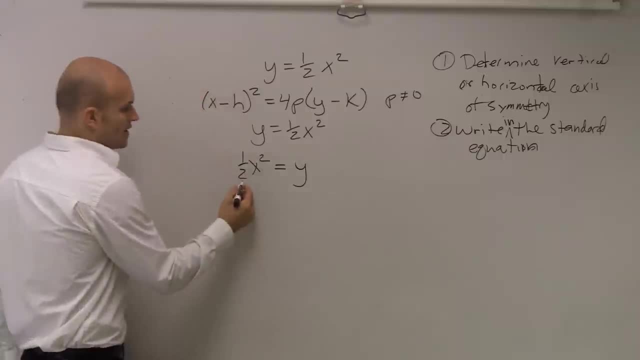 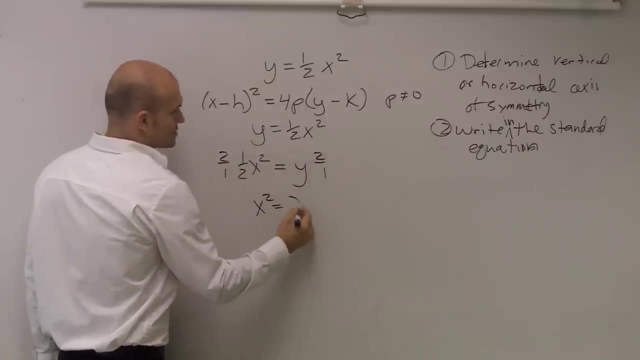 And then there's nothing always in front of there. so let's get rid of this 1 half. So what I'll do is multiply by their circle. So therefore I have x squared. All right, So you're going to get the x squared. 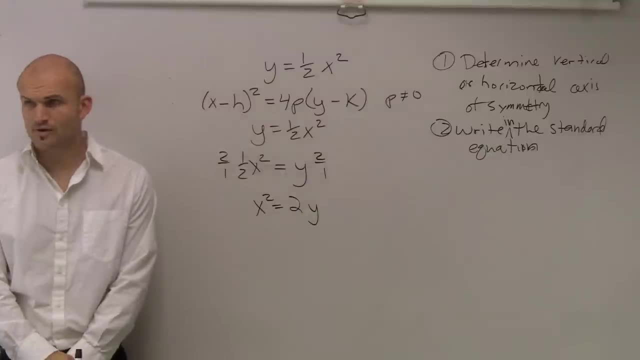 So I'm going to put this in the form. Here's the first of those two. So what I'm going to do is I'm going to write this: x squared equals 2y. Does everybody follow me so far with what I did? 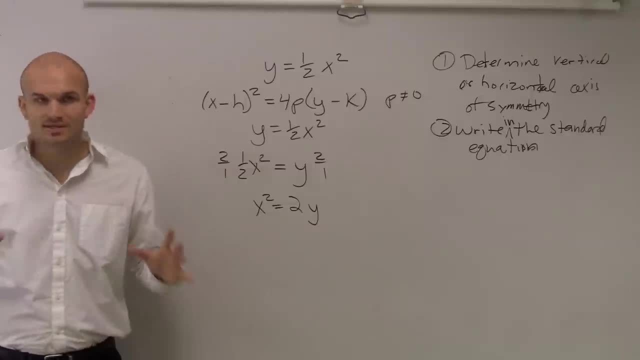 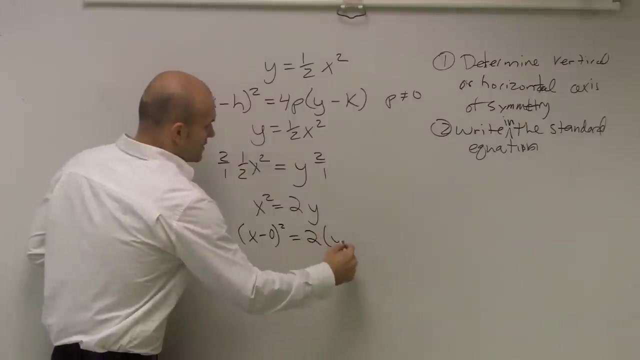 So far, yeah. Okay Now for the purposes of this problem, just since this is our initial problem, I want you guys to understand that our h and k are 0. So I could write it like this: x minus 0 squared equals 2 times y minus 0 squared. 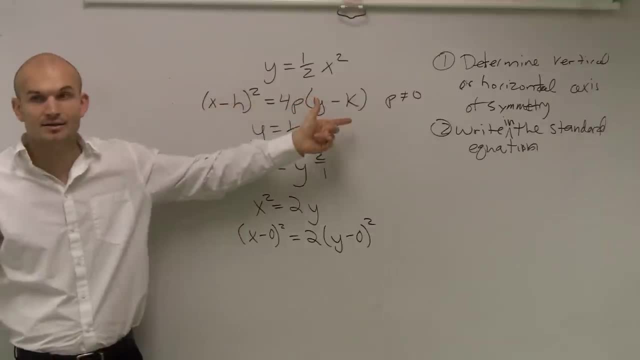 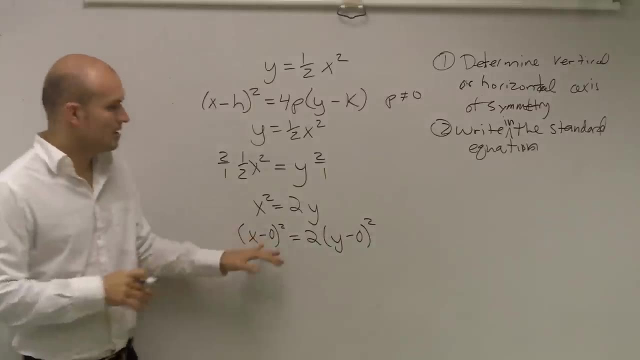 We are going to have problems where our vertex, our h and our k- okay, OK, our vertex, which I have written up there vertex, is h comma k. We are going to have problems where h or k are going to be numbers. 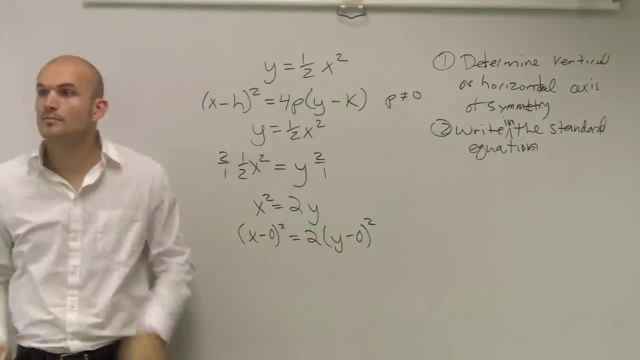 OK Square on the second side. So are you going to tell us that they don't? Huh, Are you going to tell us, Yeah, and when you have a problem you'll be able to notice when you have a different vertex? 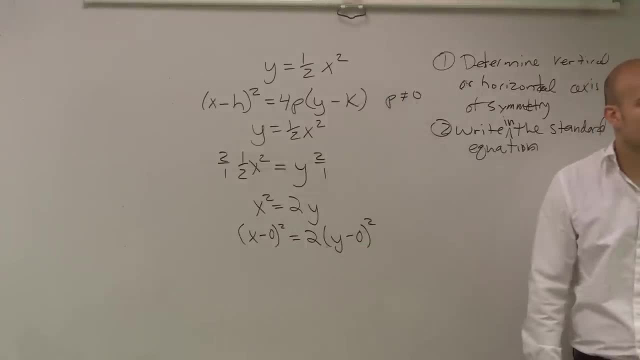 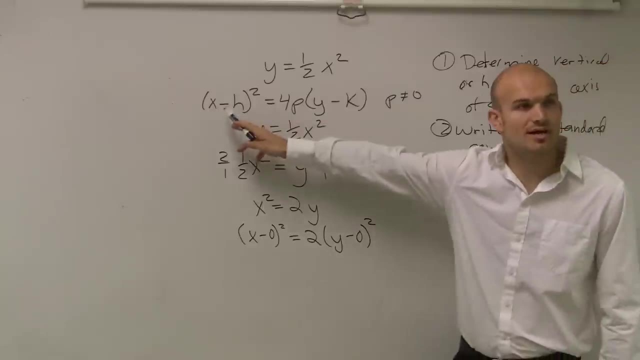 But for right now I'm just writing it, so it looks exactly like this problem. All right, What's different Square on the second is you put a square, you see? Yeah, that's what I want to try on the other one. 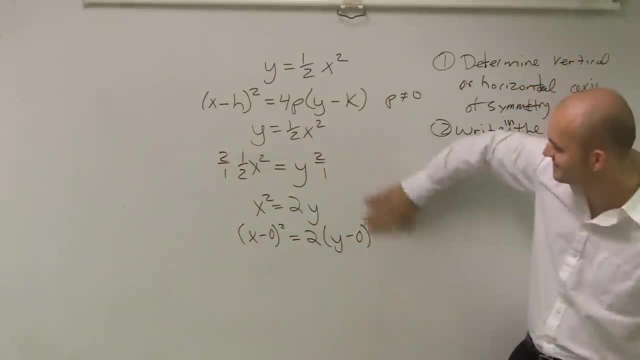 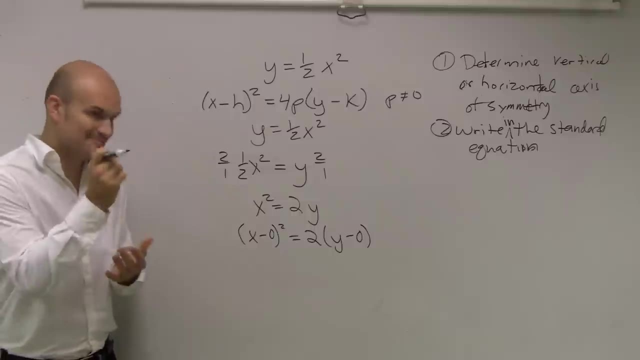 No on the second one. Yeah, on both sides, Both sides. OK, Oh, I see, Sorry. Yeah, I was just counting it. So yeah, you have 2 times your y minus 0.. Thank you. 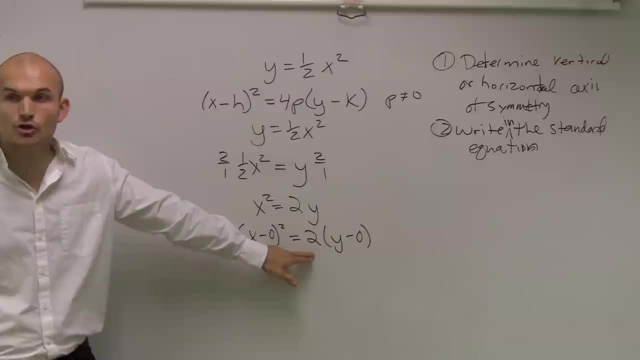 I appreciate it. So now the next thing is this: 2. What does the 2 represent? The 2 is this number equals that 4p, right? So what I can say, then, is: 2 equals 4p. So what exactly is my p? 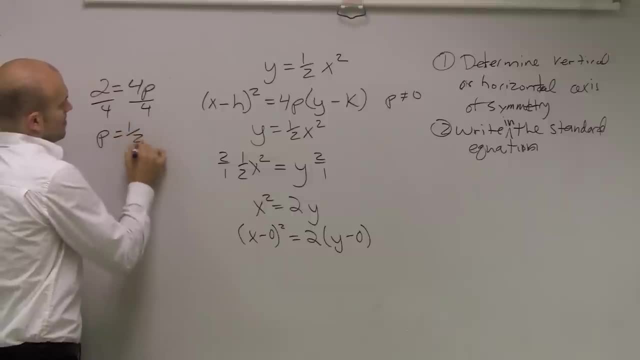 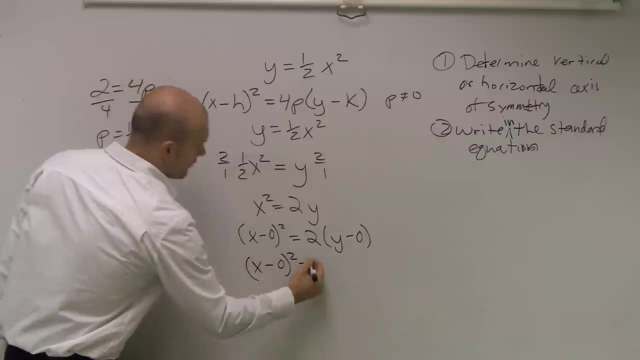 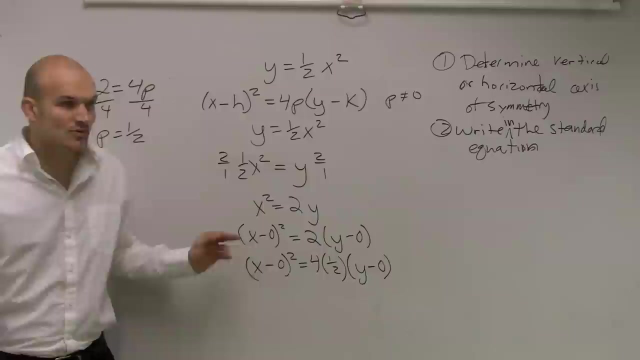 Well, 5 by 4.. 5p equals 1 half. So what I have is x minus 0 squared equals 4 times 1, half times y minus 0.. Now do I have every single component? Like I said, I've played numbers. 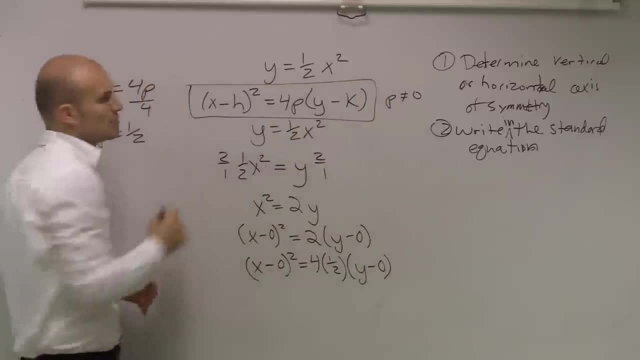 That looks exactly like my standard equation. Do I have all the components now? Yeah, I do. All right, So let's just so then. all I'm going to do now is so. I wrote it in standard form. Now I'm just going to um, this number is in the spot of this: 4p. 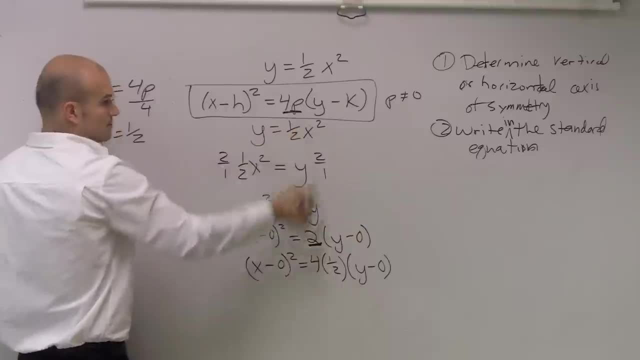 right. So 4p equals that. So you just write: 4p equals that number that you're multiplying by your y. So I solve for p to get p equals 1 half. And the reason why I want to do that? because I want to know what p is. 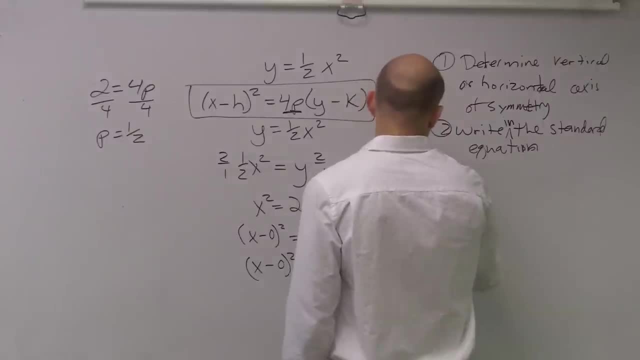 and I'll explain why in a second. So the first thing is our vertex. Vertex, remember, is your hk. It's 0, 0.. You guys don't need to write the x minus 0, the y minus 0.. 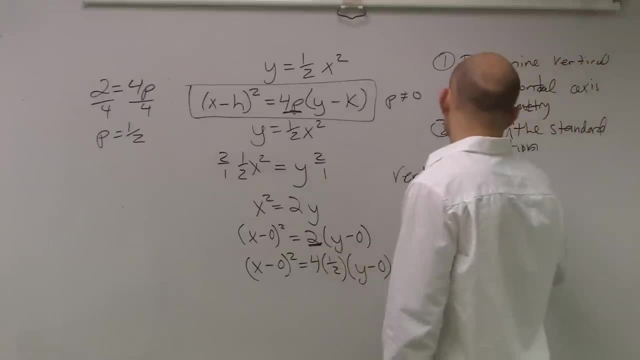 But I wanted to show it to you, at least for this first problem. so you can see that you're going to have 0, 0 as your vertex. All right, If you already have it in this form, you can just say hey. 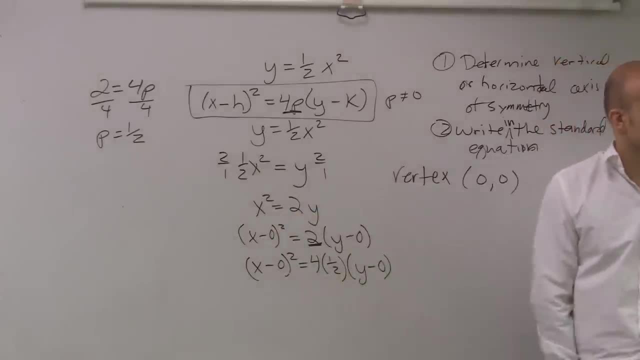 oh, you're not minusing anything, so it's 0, 0.. Right. The next thing is we need to figure out what the focus is. So the one thing with our problem is now we know it's a vertical parabola with a vertex at 0, 0.. 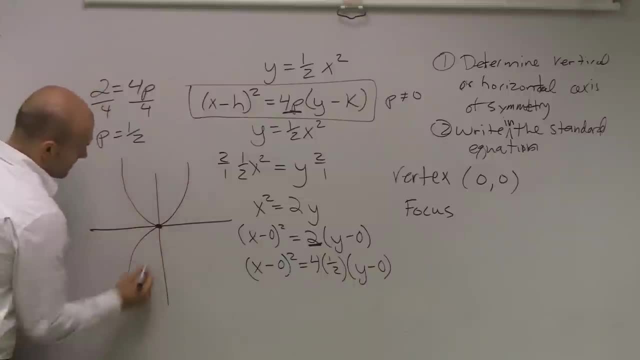 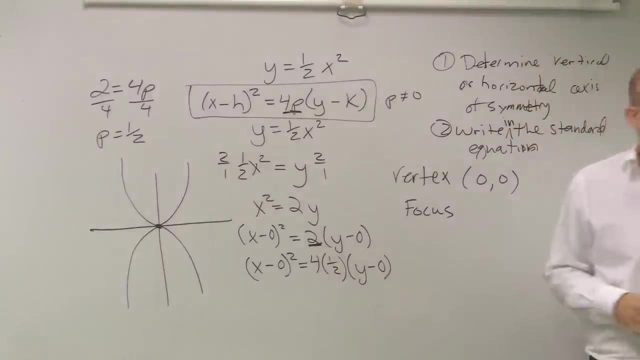 So my parabola either goes up or it opens down, All right, And without even doing it, I can't stop kind of thinking: let's take a look at what is our. how are we going to figure out our focus? Our p is 1 half. 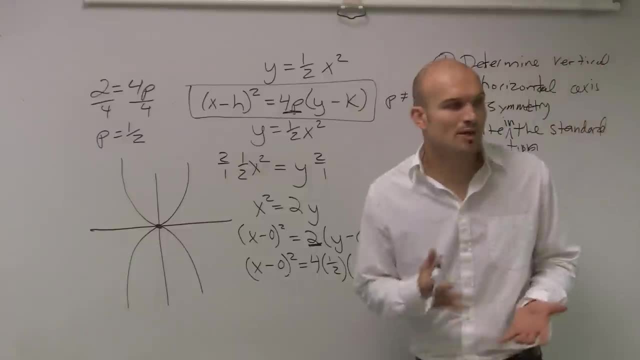 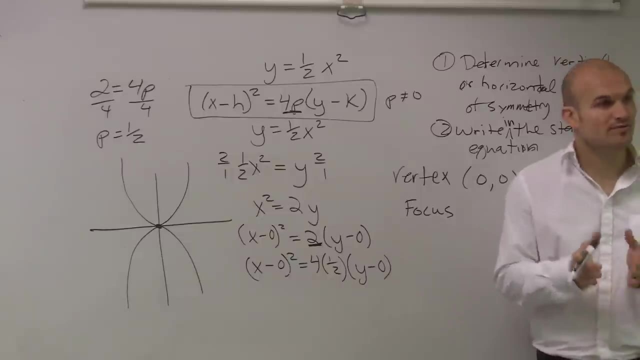 And what exactly is? what does p represent? p represents your distance from your vertex to your focus, And it also represents the distance from your vertex to your directrix. So if my p is a positive 1 half, that means I have to go up. 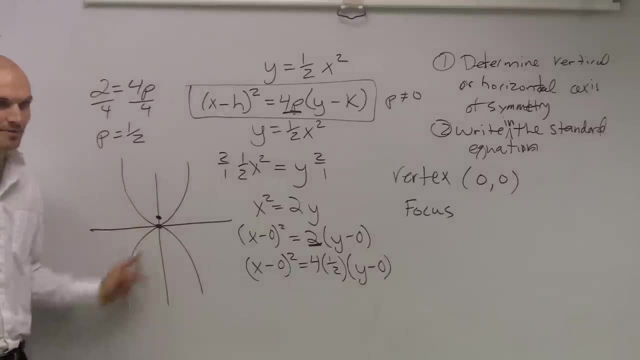 Right. So then could it be possibly this parabola? Could that be my parabola? No, Because p is 1 half, So it has to go up. It'll be 4 for a while. It'll be 4 for a while. 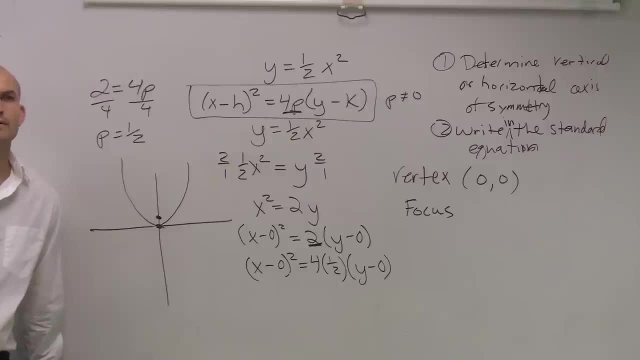 What's that? It'll be 4.. 4.. It'll be 4.. 4 times 1 half. Yes, That's just part of the formula. Your p, though? it's 4 times p. p is the distance from your vertex to your focus. 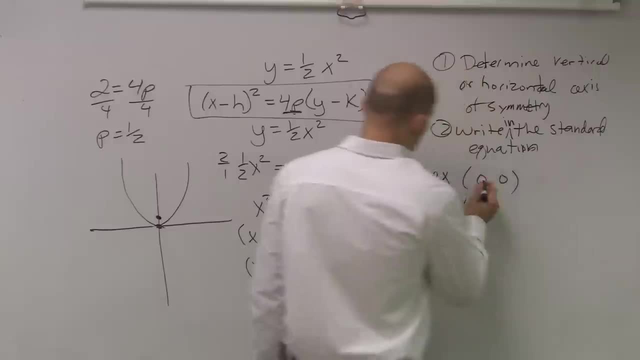 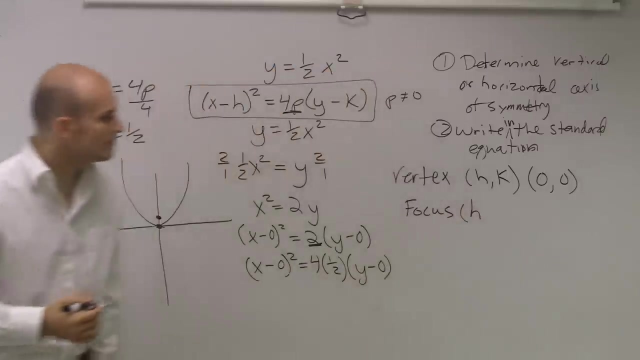 OK, And here's how we figure out your vertex. I should probably write out the formulas for you. Your vertex is h comma k, which in this example was 0, 0.. Your focus for a vertical parabola is h comma k plus p. 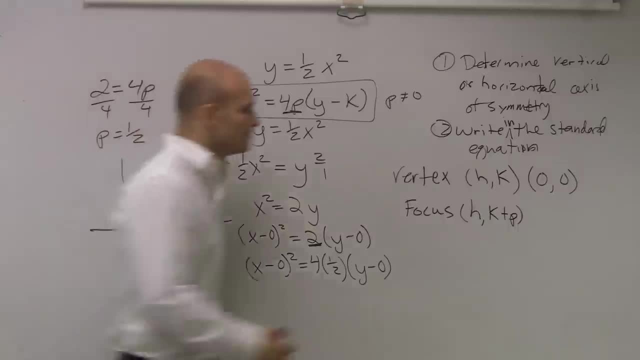 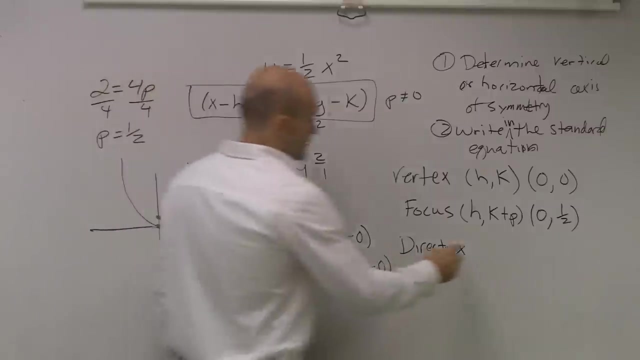 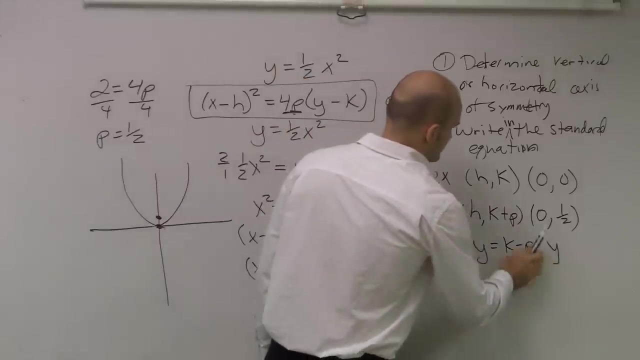 And that's for a vertical one, because obviously it's going to be dealing. It's going to be dealing vertically, which in this case is going to be 0 comma 1 half, And then the last one, the directrix is going to be: y equals k minus p, which equals negative 1 half. 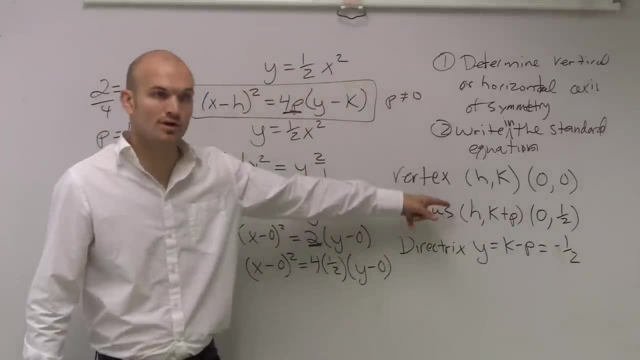 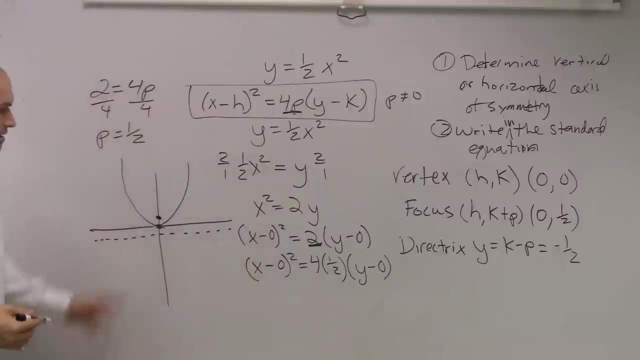 It's not a point. It's not a point. Directrix is not a point. Our focus is a coordinate point. Our directrix is a horizontal line in this case, Because, remember, our directrix is just the distance. It's going to be automatically distant. 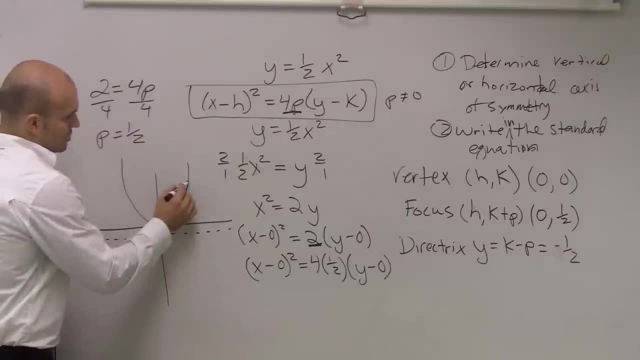 Whatever it is from your focus that distance makes up all your points, These distances are the same. OK, So from your focus to any point on the parabola back down to the directrix is always going to be the same, All right. 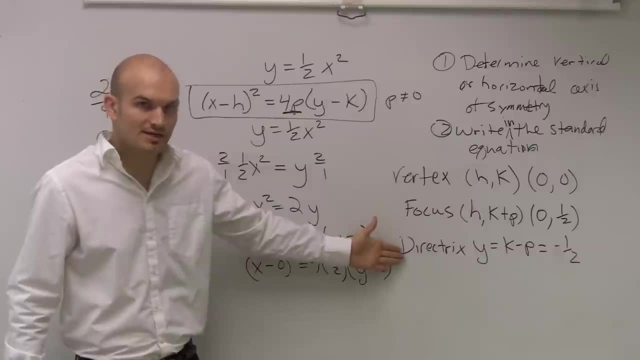 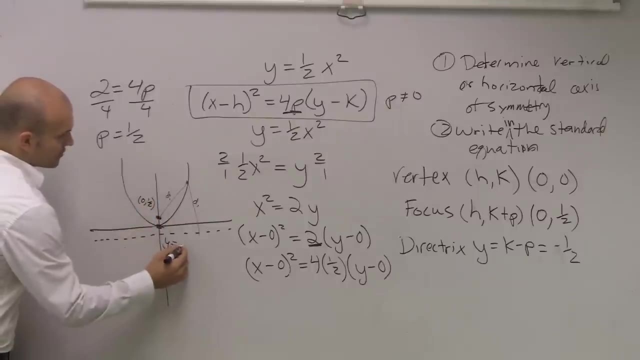 So now I've determined what the vertex, the focus and the directrix is. You guys can see: my focus is at 0 comma 1 half. My directrix is: y equals negative 1 half And my vertex is at 0, 0.. 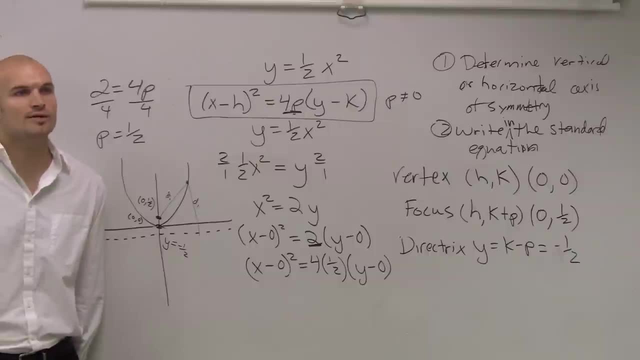 So now I've just completed just a rough sketch of those kind of three important points to make my parabola: Yes, So the directrix is going to be the same as p, but in the other way, The opposite. It's the distance from your vert-p. 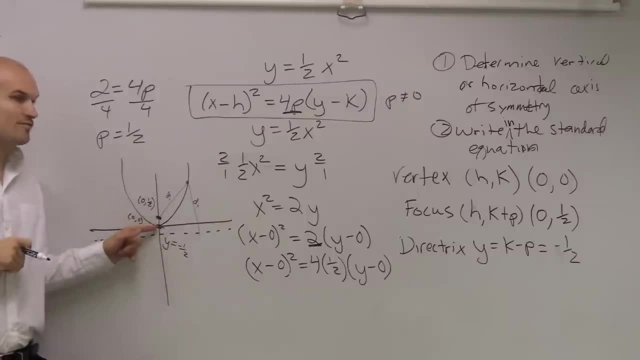 p is the distance from your vertex to your focus and to your directrix. OK, OK, So what we're doing when it's vertically, if you're adding p to find the focus, then you have to subtract p to find the directrix.